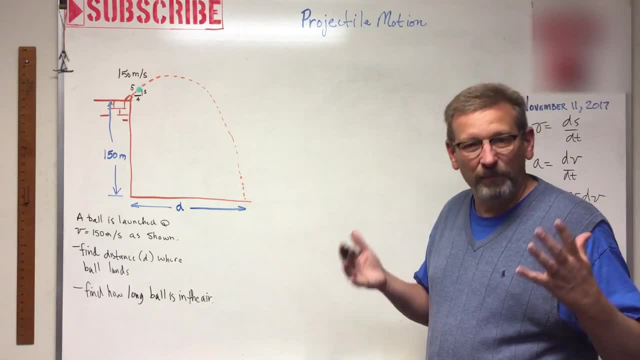 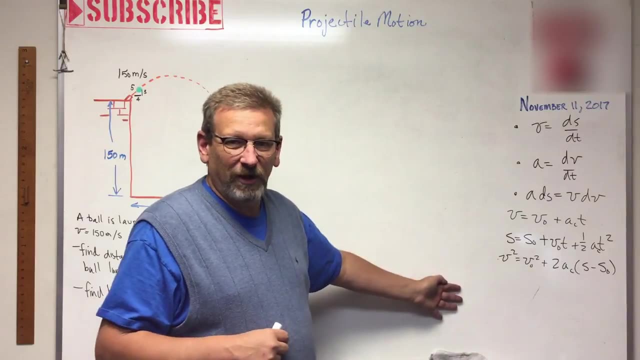 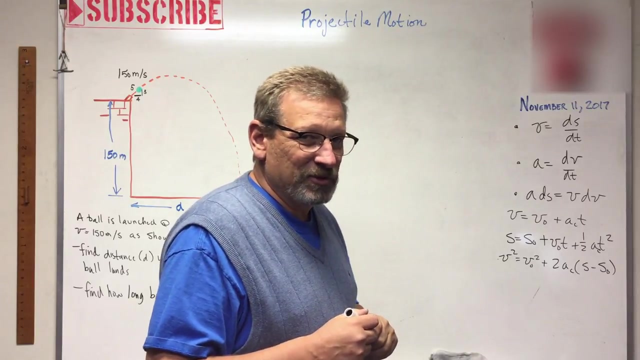 FE exam, or you know. it's just a very common problem that's worked out in dynamics And it's not too bad. We're going to use all of our old equations that we derived in our last video on constant acceleration, Because you know the funniest thing about projectile motion. 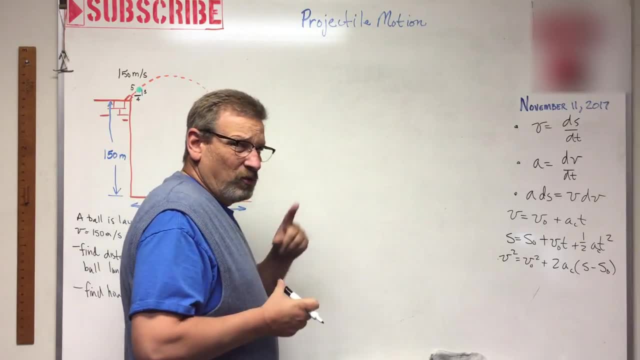 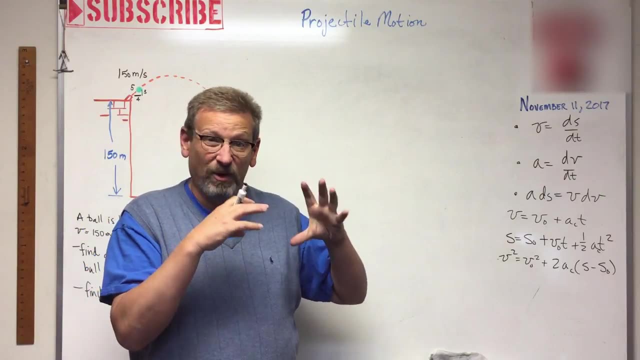 it's not funny, but I guess. but is there's only one acceleration at work Once? if you have something like if you shoot a bullet out of a gun or a cannonball out of a cannon, there's only one thing once the projectile leaves the muzzle of your gun or the cannon. 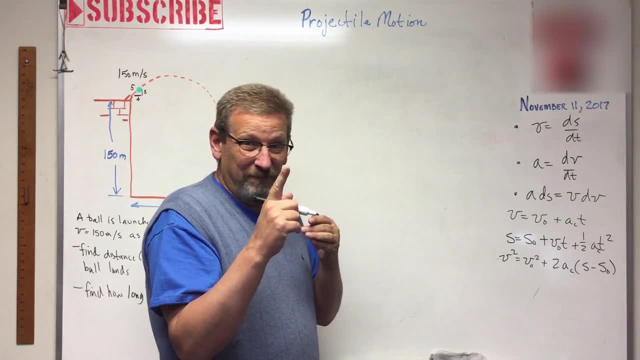 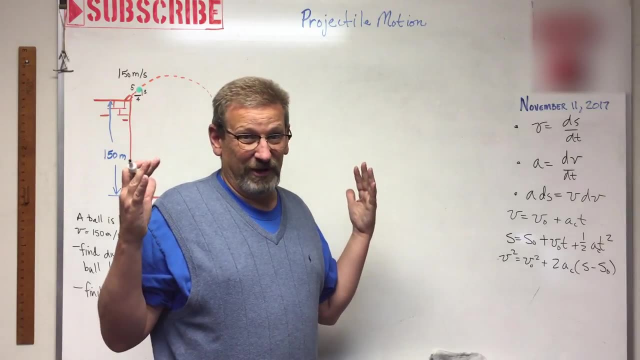 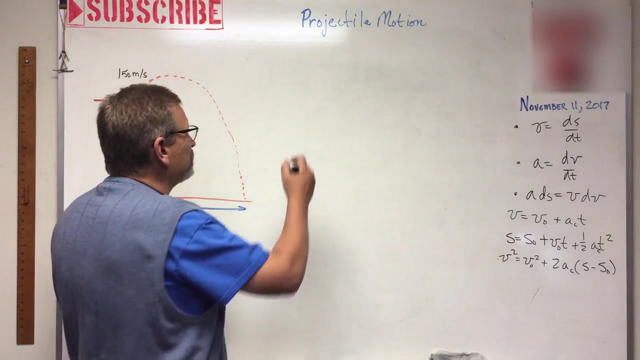 there's only one thing accelerating it. It's not gunpowder, It's gravity. That's the only thing there is. So it doesn't. once it leaves the barrel, it's never, ever going to get any faster. Okay, So there's a couple of things that you need to know about projectile motion. Number one: 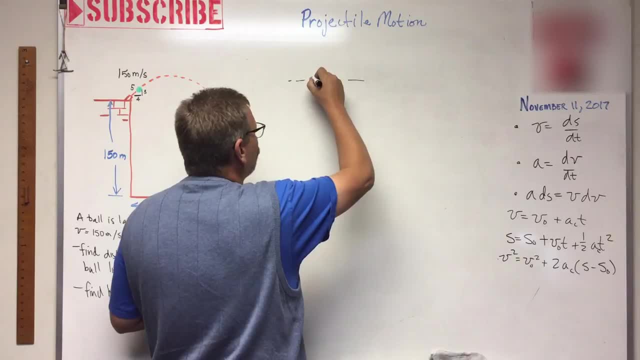 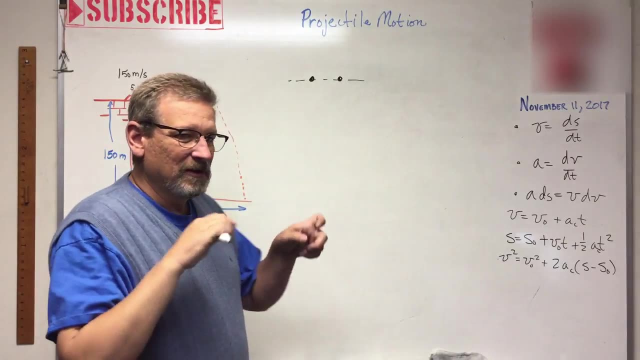 is if I have something and I from a datum here, if I drop something and I have something over here that I have maybe shot at the exact same time. So I had a, a switch and the end of my gun and as soon as the bullet passed, it dropped a projectile at the same time. 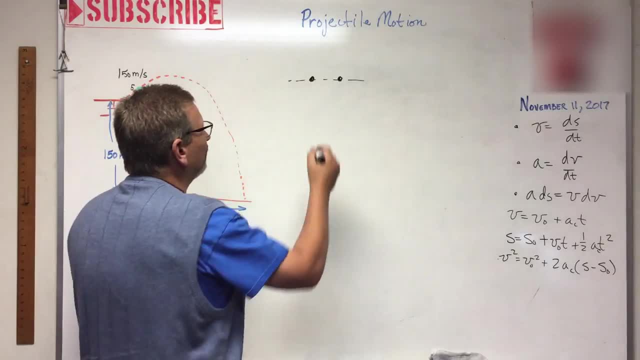 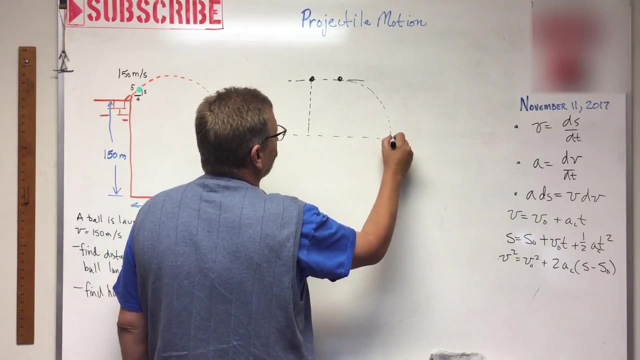 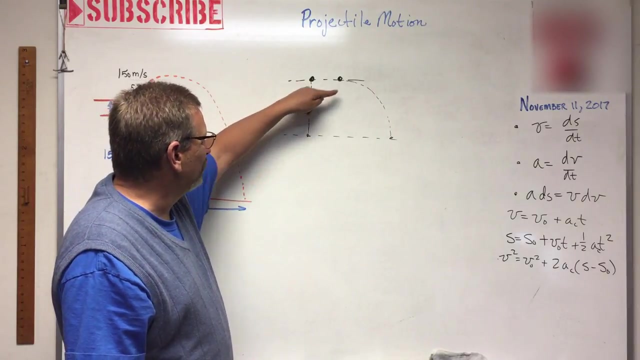 one was going out. Okay, So those two are going at the same time. Guess what? As this one goes out, it falls, And as this one falls, they both fall and they will both hit the ground at exactly the same time, because this one is being accelerated by gravity downwards, And so is that one. It's 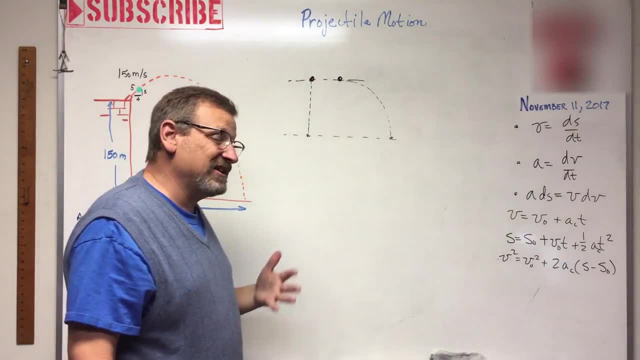 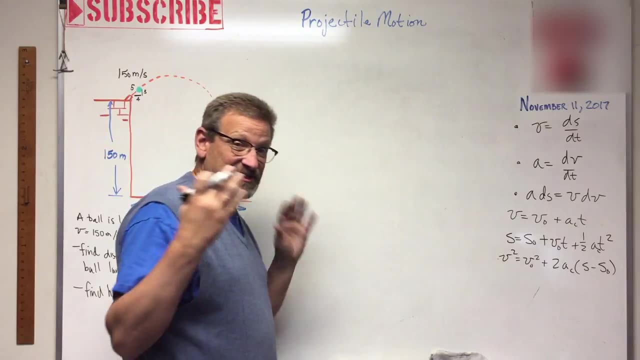 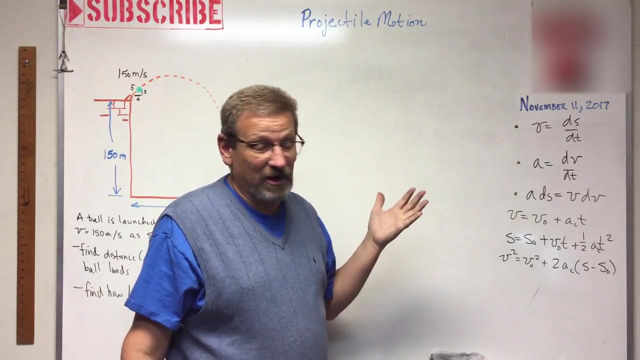 not being accelerated forward anymore. So that's something you need to know about projectile motion. Okay Now, projectile motion, since gravity is the only thing that's working on it. of course, acceleration is going to be constant all the time. So if acceleration is constant, we can use. 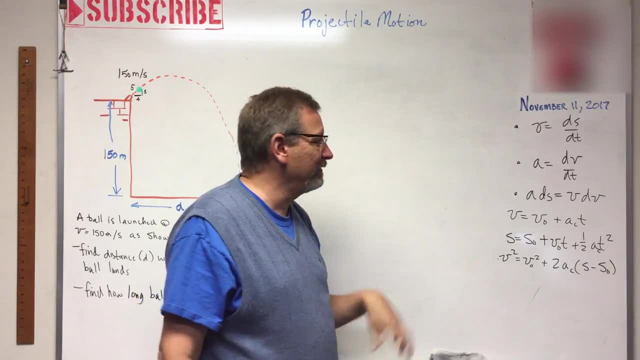 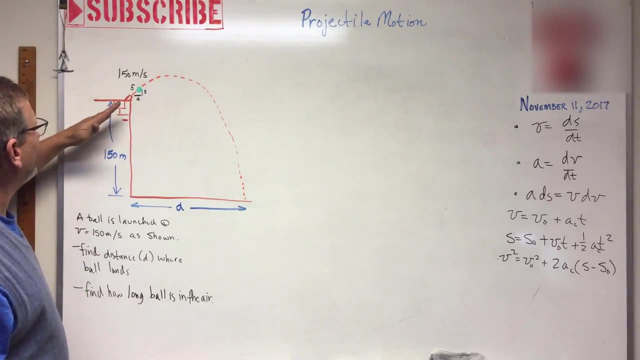 our constant acceleration equations that we've been, that we've derived in the last video. So let's look at this little problem here. So we've got a building- it's 150 meters high- and we've got some- I don't know. it looks like a tennis ball launcher and it's going to shoot a tennis. 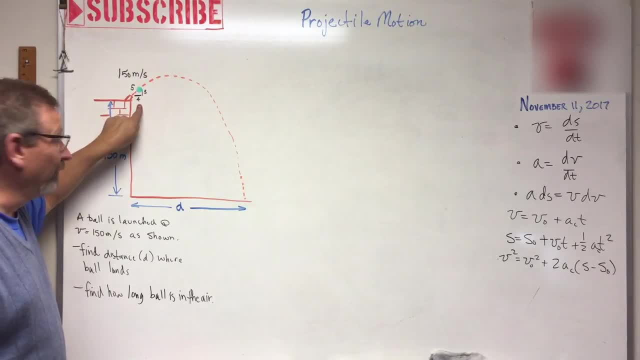 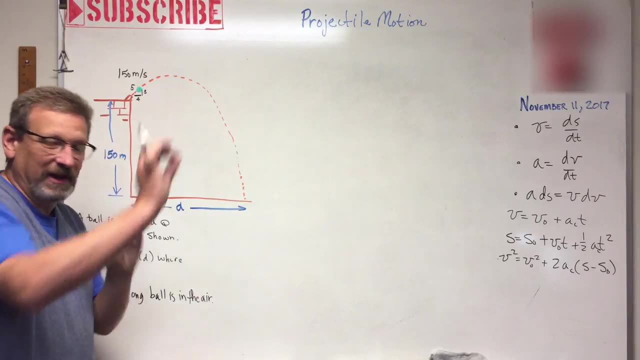 ball at an angle. It looks like a tennis ball launcher And it's going to shoot a tennis ball at an angle. It looks like a three, four, five triangle, doesn't it? And it's going to shoot it at 150 meters per second. So that's the velocity when the projectile leaves the barrel, Okay, And 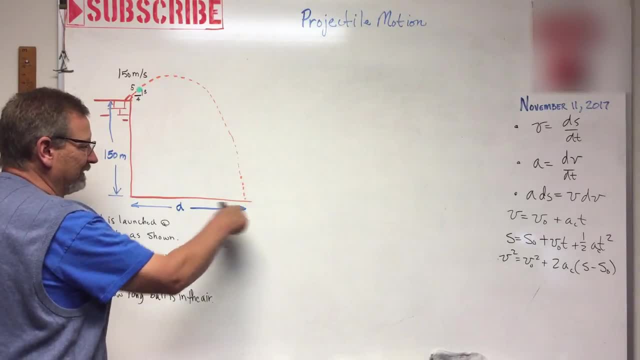 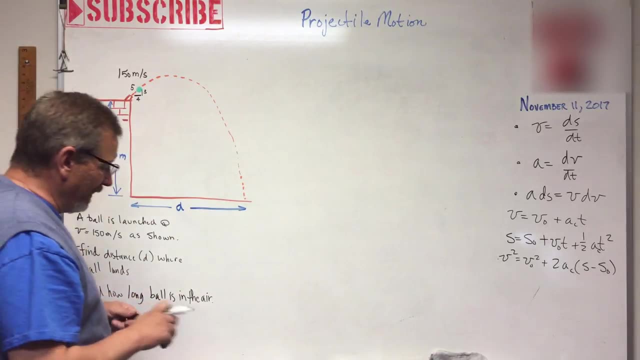 they want us to find the distance where the ball lands. So what is D? What is that distance there? And then, how long was the ball in the air, right, How long was it traveling? Now you got to. the way you think about that is this: You think about these equations in two directions. So, just like, 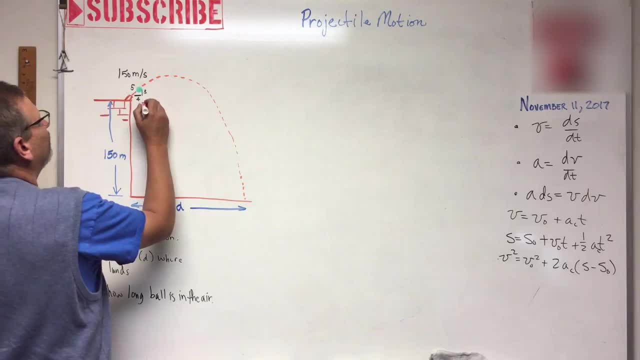 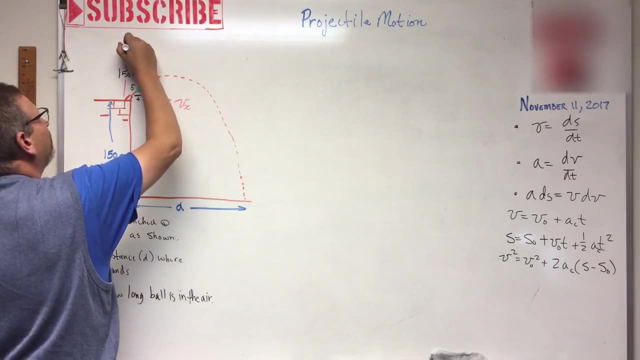 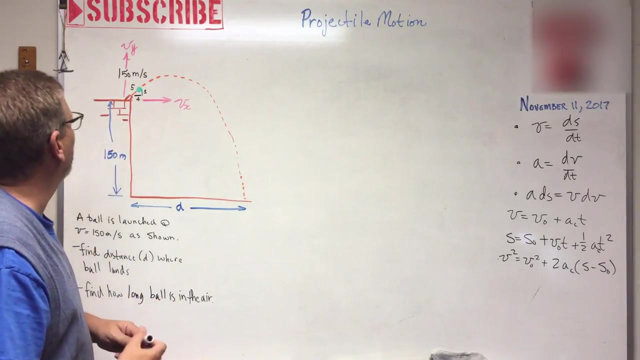 I said we can break it into X and Y components. Okay, So we have like: here we have the velocity in the X direction, And then here I have the velocity in the Y direction. That marker's pink. Okay, And so in the X, what is the acceleration going to be? 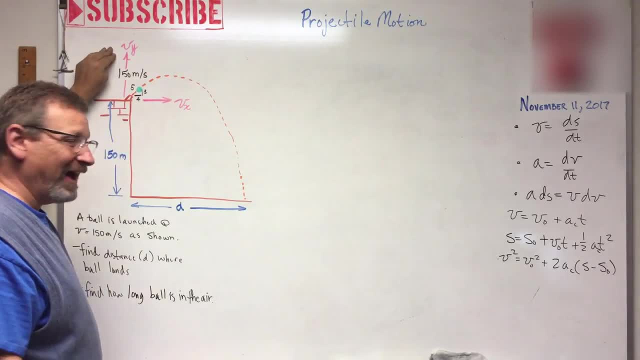 Zero. There's no acceleration in the X. How about in the Y? What's the acceleration going to be? Ah, that's where gravity lives right in the Y direction, because gravity sucks right. So for a problem like this, we can take these equations and solve it. So I think you know, I know the. 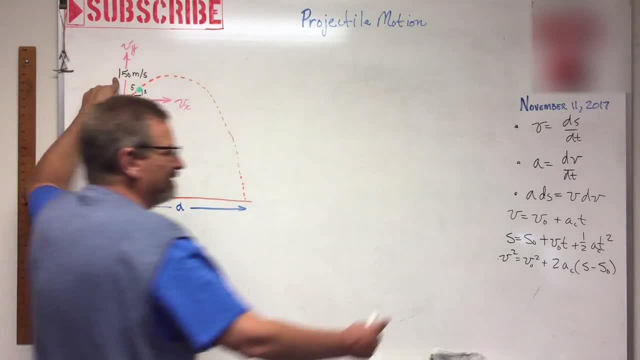 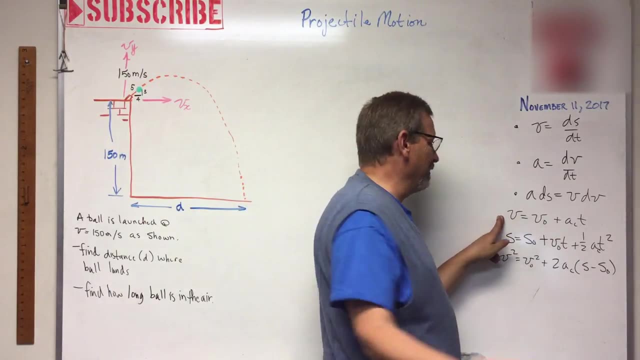 initial velocity but I don't know the final velocity. So that kind of rules out, that equation. I don't know this, you know. I don't know. I don't know the time, I don't know how long it was in the. 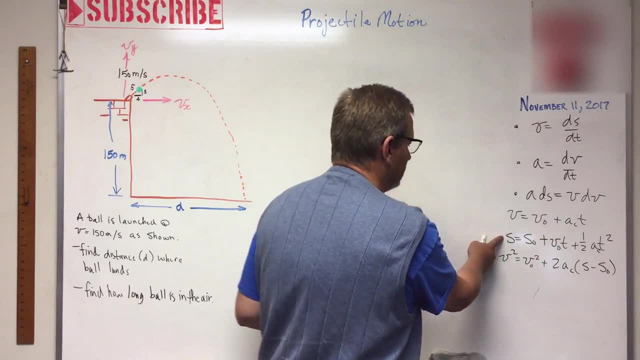 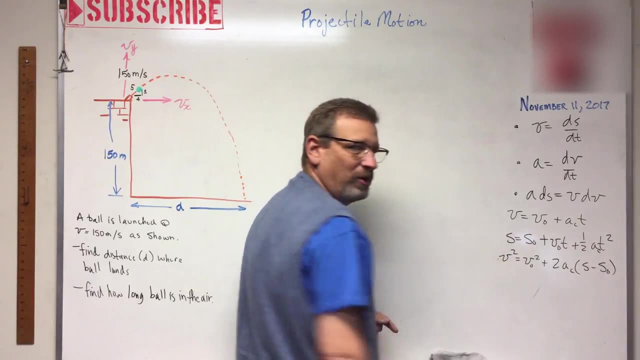 Air Force That has too many unknowns. But look at this equation. I know where it starts out, I know where it finishes, I know what the initial velocity is And I know where it finishes And I know where the acceleration is. The only unknown in that equation is going to be T. Let's use that one. 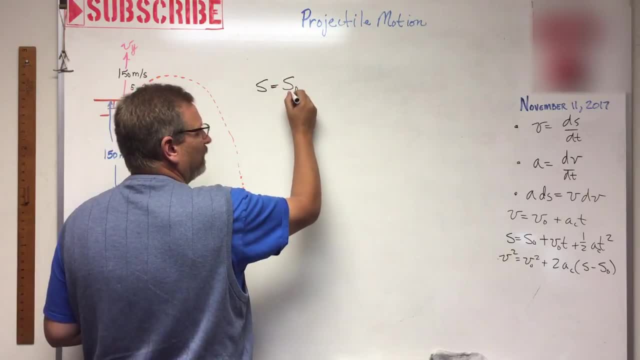 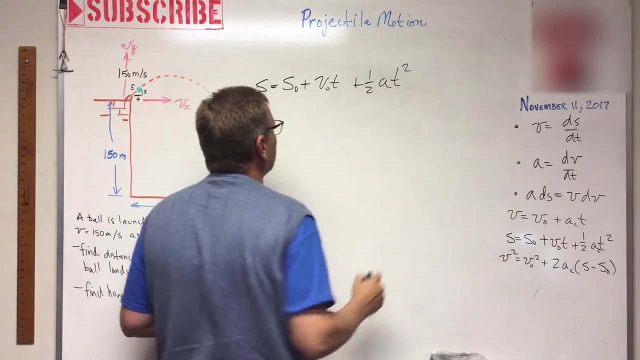 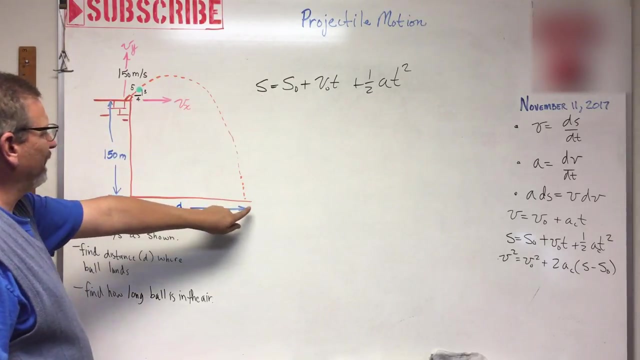 Okay, So S is equal to S. naught plus V, naught T plus one half A T squared. Okay, So let's just substitute in what we know. So S, of course, is final position. Let's call that zero, right, He's. 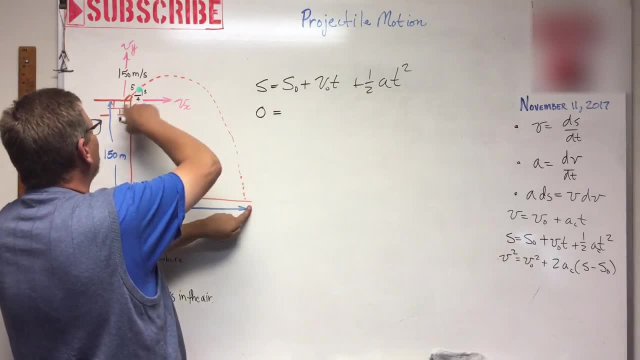 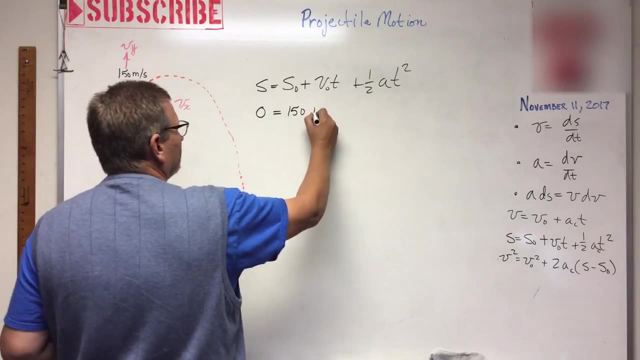 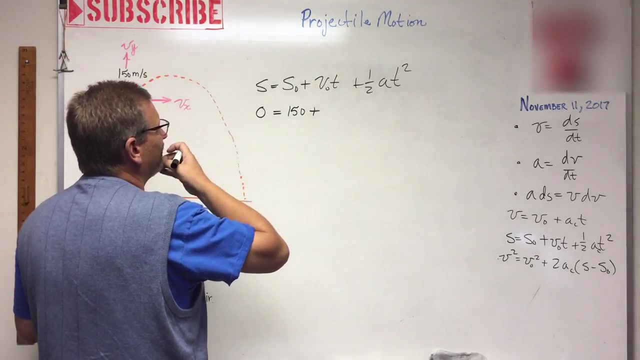 going to wind up at zero. Where did he start out at? He started out at 150 feet off the ground, Because that's how tall my building is over here, Plus all right. now, what are we doing here? Let's do, let's do this in the Y direction. Okay, This is in the no, this would be in the X, right. 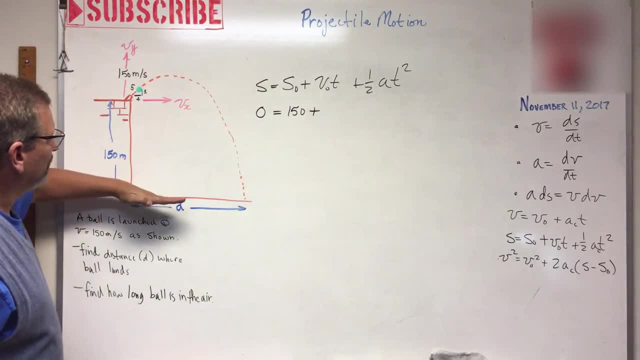 No, that's Y, isn't it In the Y direction? our final position is at zero. Our initial position was at 150.. That's the Y right, And so we're going to use this right here. Okay, So the initial. 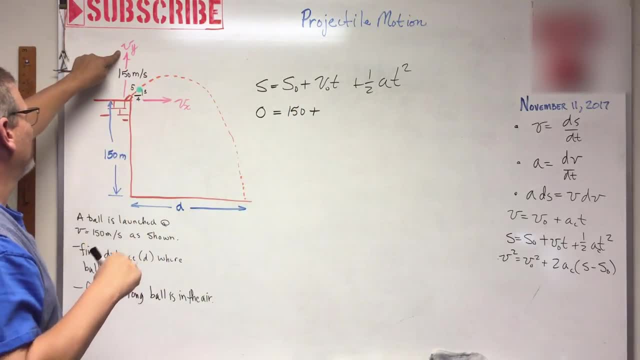 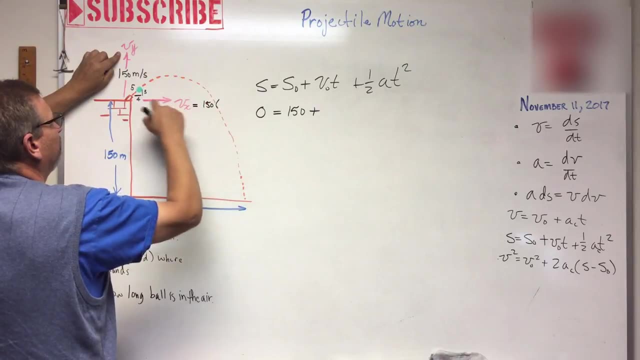 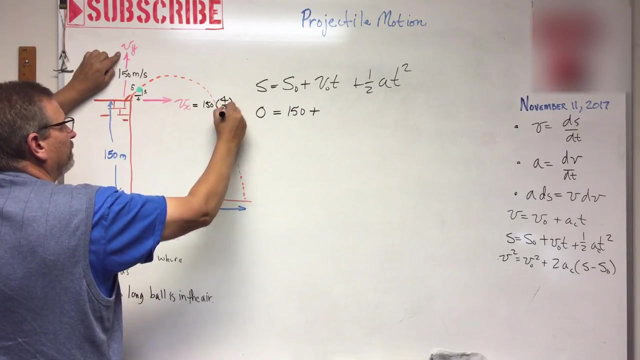 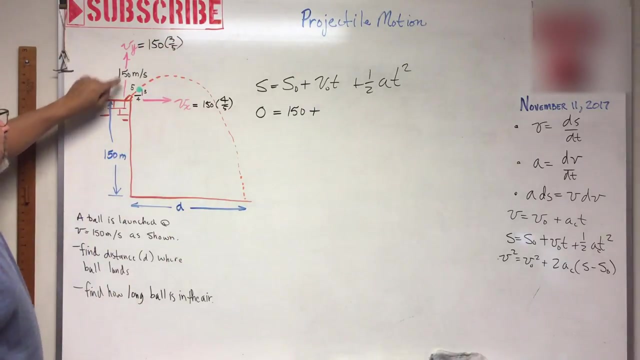 velocity was was 150.. But what is this component? Well, this one over here is, if you remember, is 150 times three. no, sorry, sorry, four over five. This one up here is 150 times three over five, You remember that. 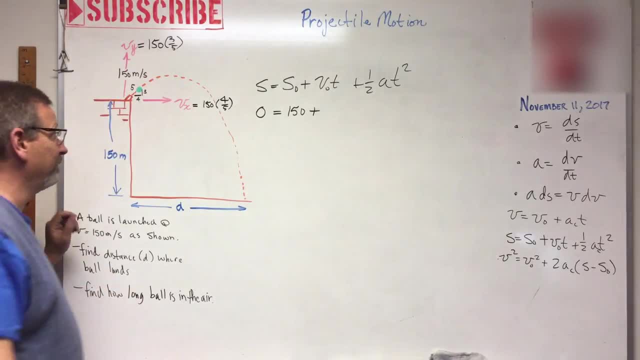 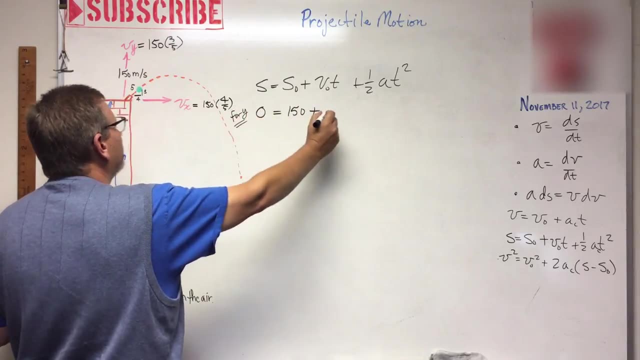 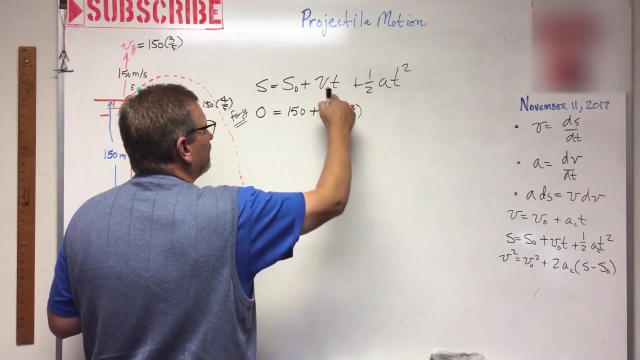 How to how to break a force into components. We should be getting good at that by now, right? So in the Y direction. this is, this is for Y, This whole equation. here In the Y, the initial velocity is 150 times three over five times T. 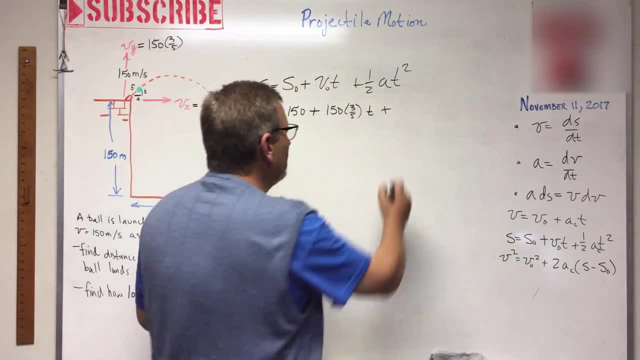 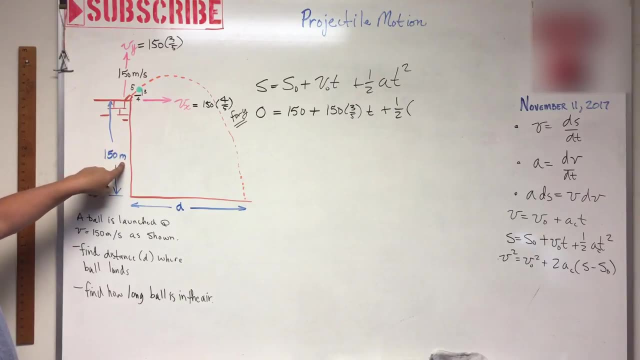 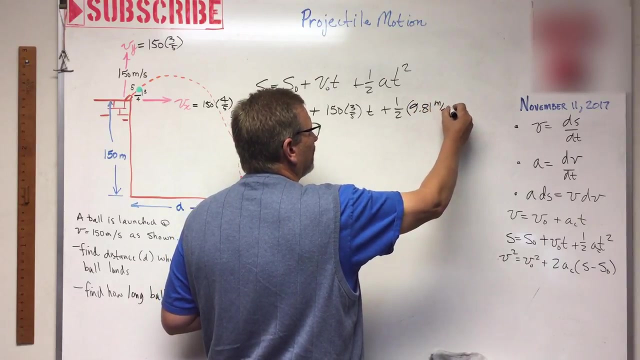 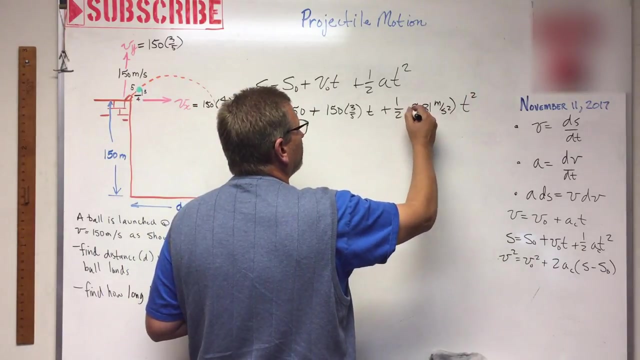 plus one half, All right. What is the acceleration? Now? this is in the, this is in a. this is a metric problem. We're in meters here. So how about 9.81 meters per second? squared times T squared? All right? Oh, let's make the 9.81 negative. So it's going down. right, All these were positive. 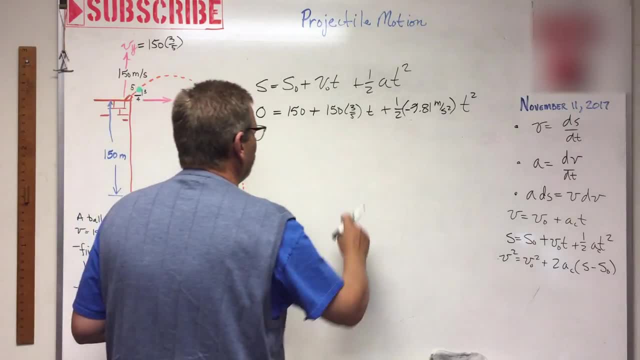 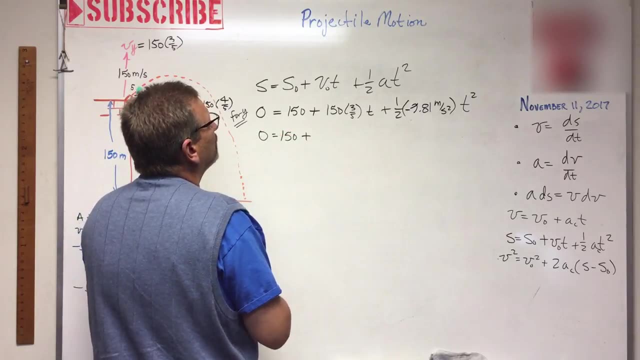 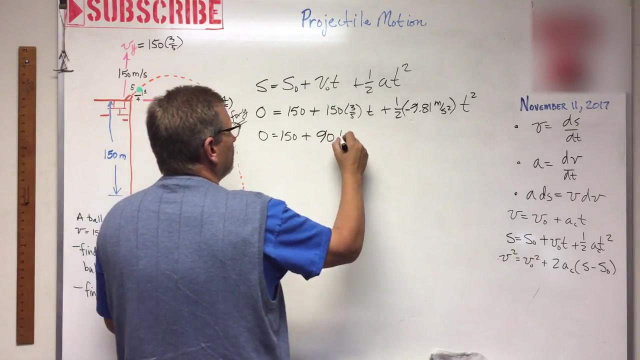 numbers. That's negative, Okay. So what do we have here? Um, this is 150 equals zero plus uh. what is that? 0.6 times 15 is 90 T, And then minus half of that is 4.97.. 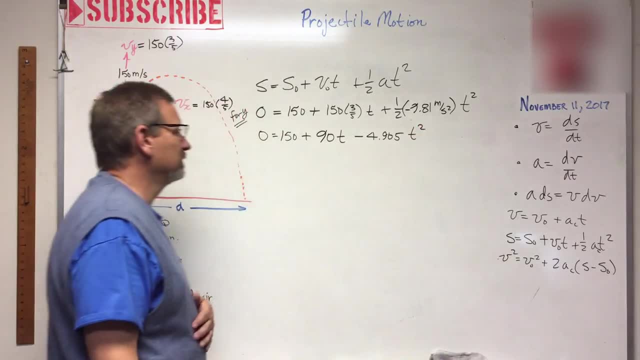 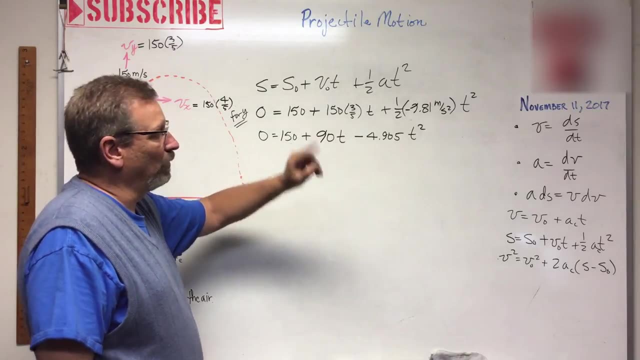 So that's going to be 5.005 T squared. Okay, Well, that's not very fun, is it? What is that? That's a quadratic equation. Oh, hang on. If you have remember, I told y'all about this. 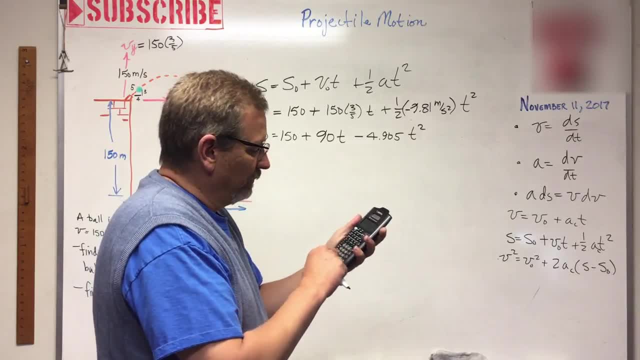 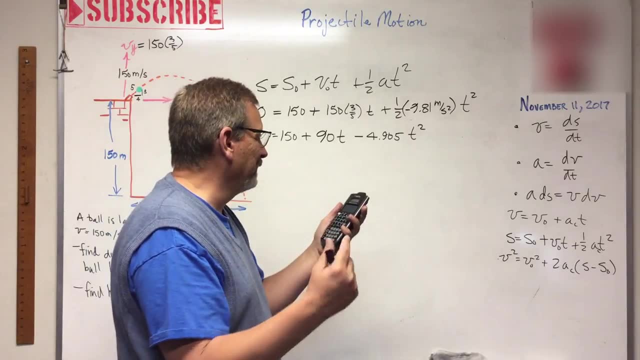 the TI-36 probe, right. If you go to on second uh polysolve: right, There's the quadratic equation. It's built in there right. I click enter and it says what is A? Well, A is negative. 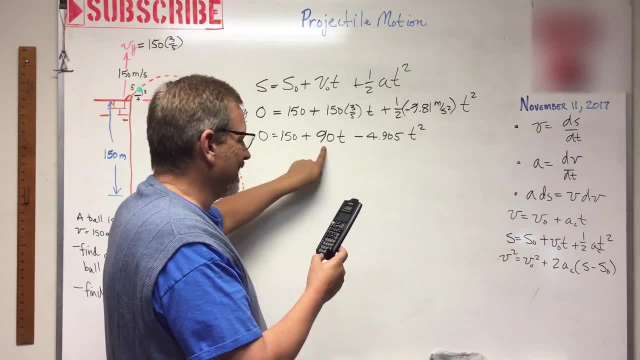 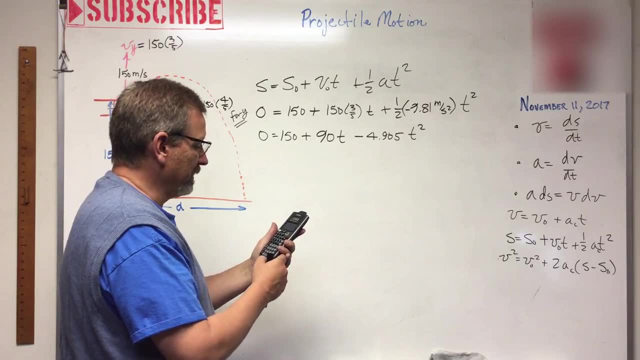 So what is A Well A is negative. So what is A Well A is negative. So what is A Well A is negative 4.905.. Enter B is 90.. Enter C is 150.. And then it says: solve Boom. I click solve, It gives me. 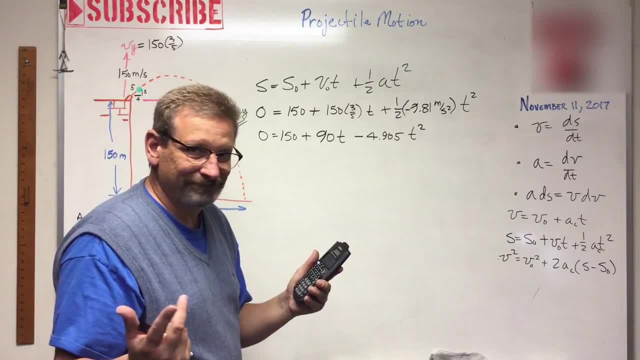 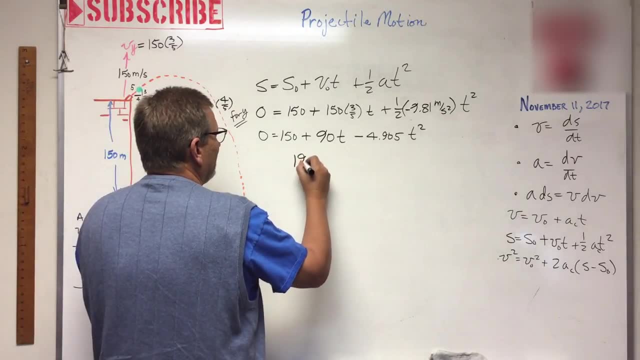 one negative root. Do you think that the time is negative? I don't. And then it gives me one positive root, which is 19.89.. 19.89.. Okay, So out of the two possible roots, only one makes sense. 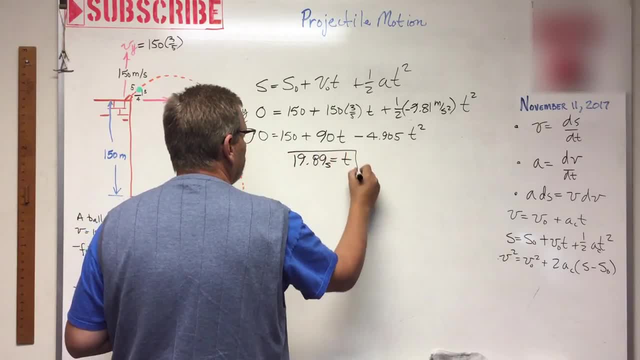 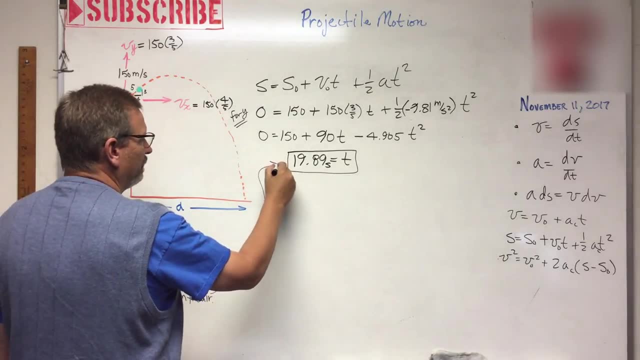 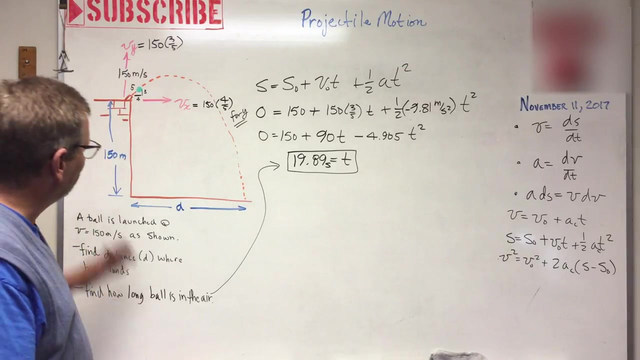 And I think that that is it, Okay. So, guess what? How long is the ball in the air? Well, it's in the air for 19.89 seconds, Okay. Well, how far does it travel? How far is it from here to where it lands? Well, you know what That? 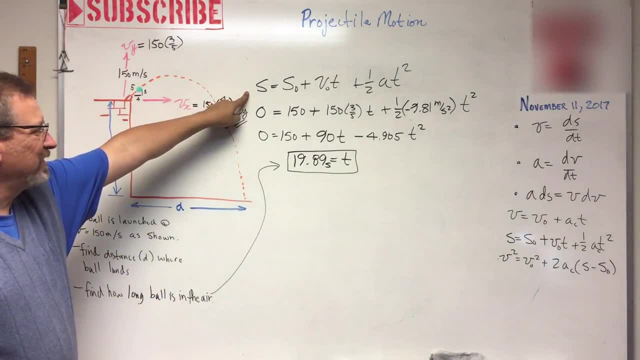 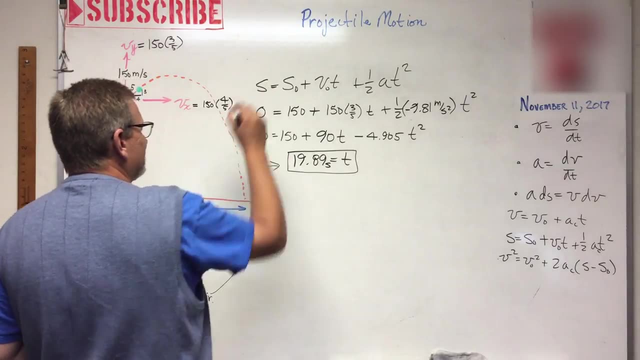 is in the X direction. So can we take the same equation and work it for the X direction? I don't know, Maybe Let's see. Okay, So S, S is the final position. You know what? That's what we're looking for, isn't it? We'll call. 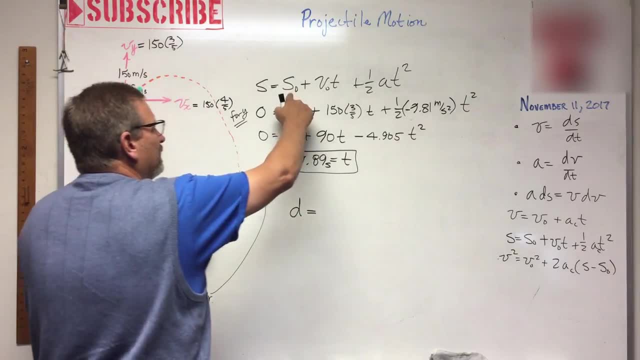 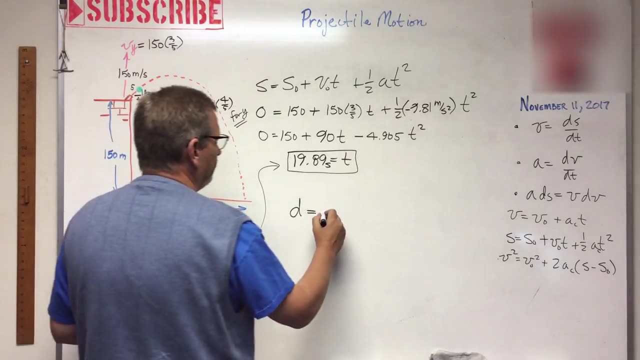 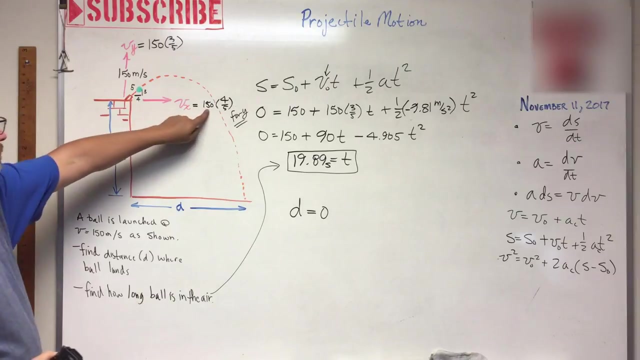 it D. D is equal to the initial position. Well, if that's final position and this is initial, then that's it. We'll call it zero. right, So zero there. The velocity, the initial velocity in the X direction, is what, Right there? So plus 150 times four over five. 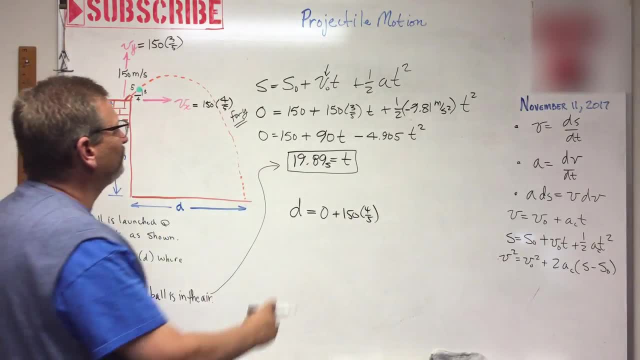 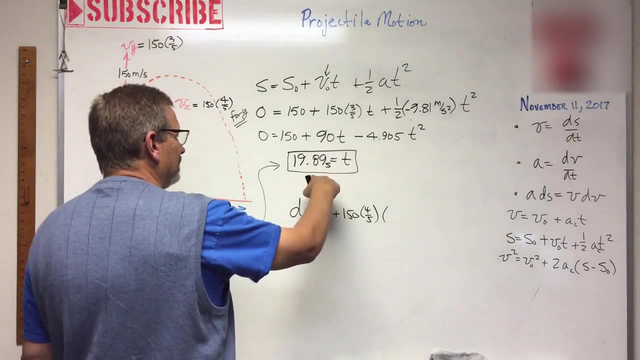 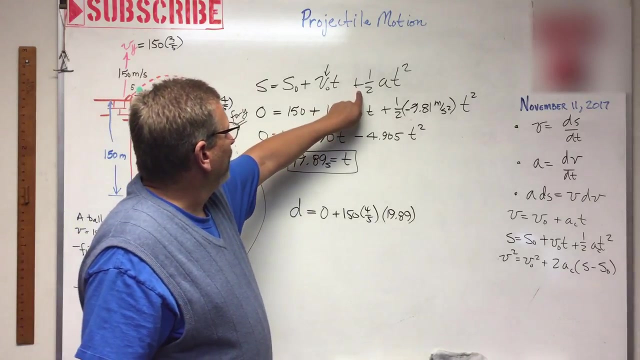 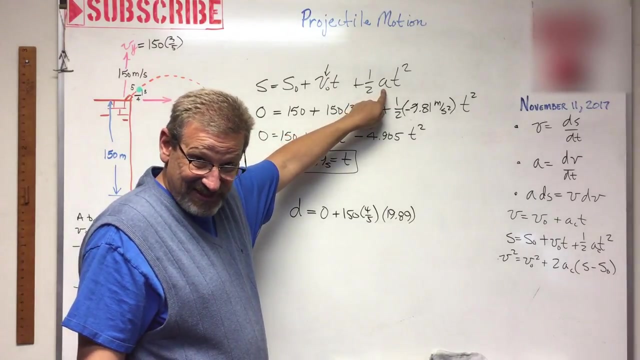 Times, T. Oh, but you know what? I know what T is. T is 19.89.. Okay, And then what Plus one half? What is the acceleration in the X direction? None, There isn't any. So this whole term here. 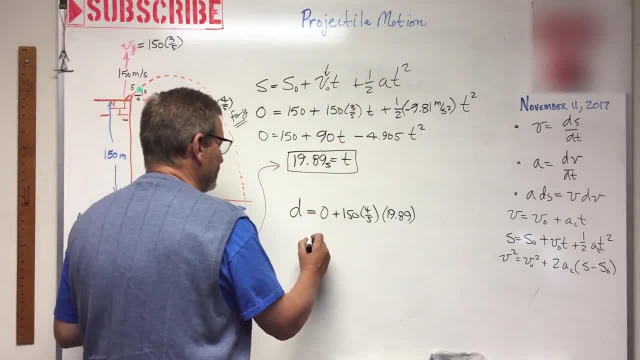 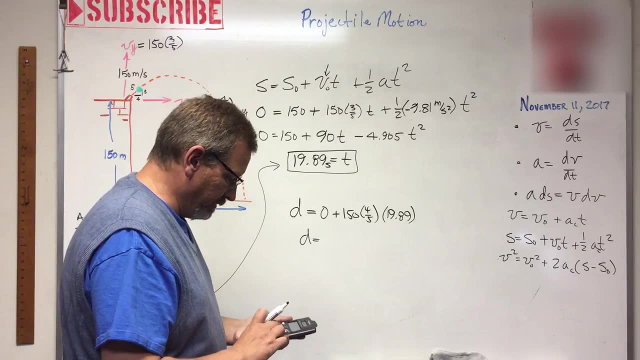 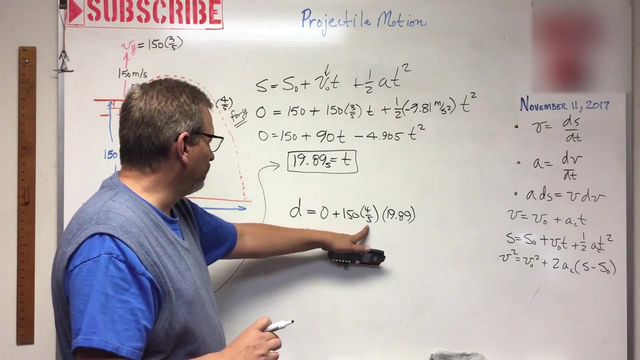 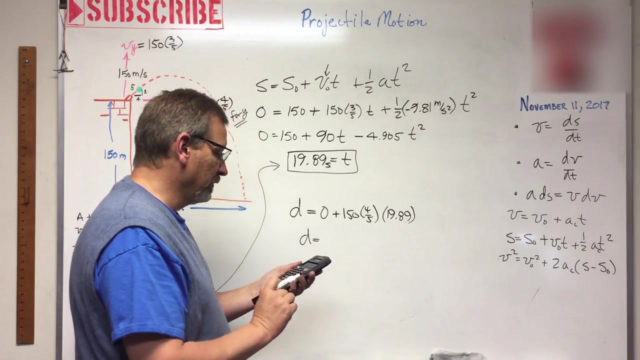 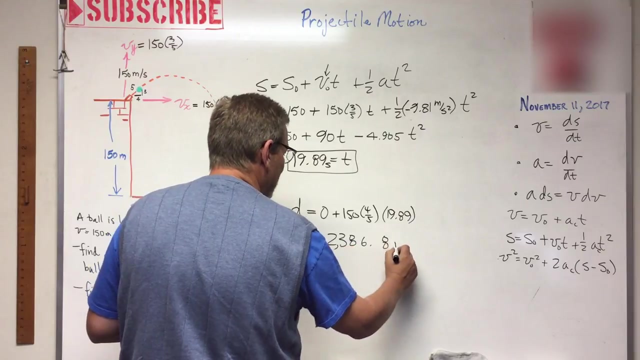 is going to zero, isn't it? Well, that's it, isn't it. So D is equal to: here we go. One Oh, clear, Enter, Clear, Okay, 150 times four, Oh times 0.8.. Let's do that, That's 0.8, right, Equals. 120 times 19.89 equals 2386.8.. And that's meters.